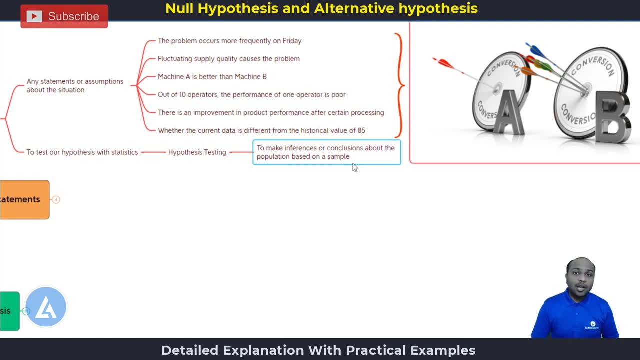 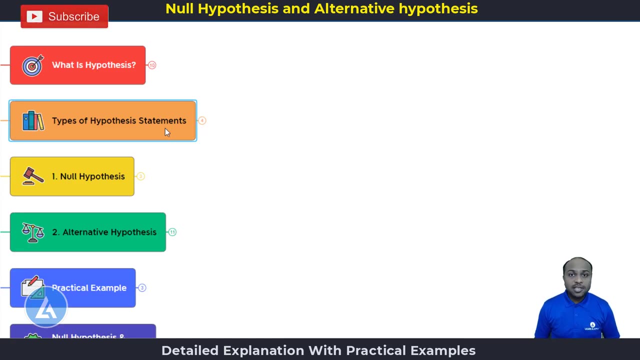 to calculate the sample statistics and the sample statistics we are going to compare with the hypothesis value to check our hypothesis. Don't worry, I'm going to explain in simple language with the help of practical example. So this is just an understanding of what is hypothesis. As we are discussing about the hypothesis testing, there are two. 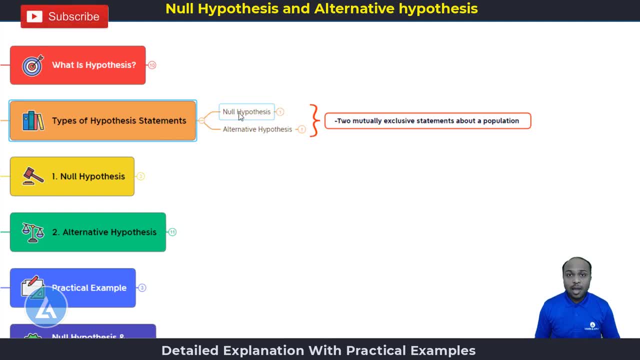 important hypothesis statements. The first one is called null hypothesis and second one is called as an alternative hypothesis. These are the two mutually exclusive statements about a population. What is the meaning of that? These two are significantly different from one another. Null hypothesis is indicated by H0,, whereas alternative hypothesis is indicated. 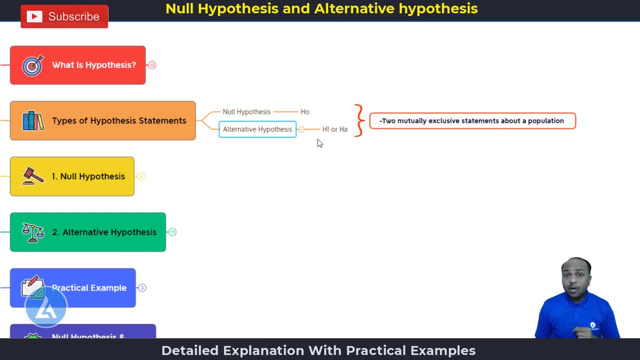 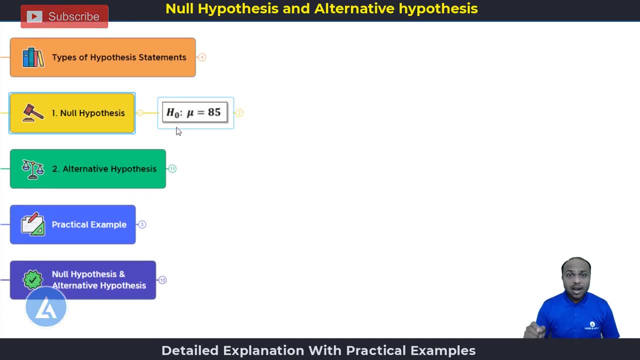 indicated as H1 or Hj. Now let's understand each of these hypothesis statements in detail. The first one is Null Hypothesis As we had seen. it is expressed as H0 and the expression will be like this: H0 colon mu is equal to 85.. I will explain this statement in detail. 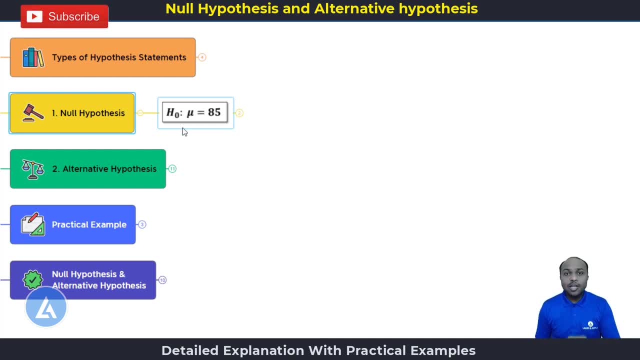 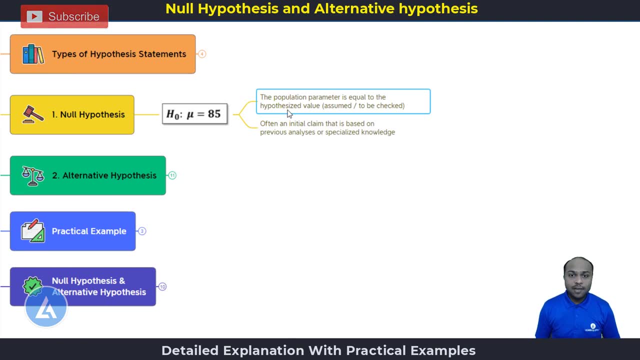 once we go for the practical example. But just understand here what is the notation. The meaning of this statement is: the population parameter is equal to the hypothesized value. Now, this hypothesized value is nothing but the value that we have assumed or that we 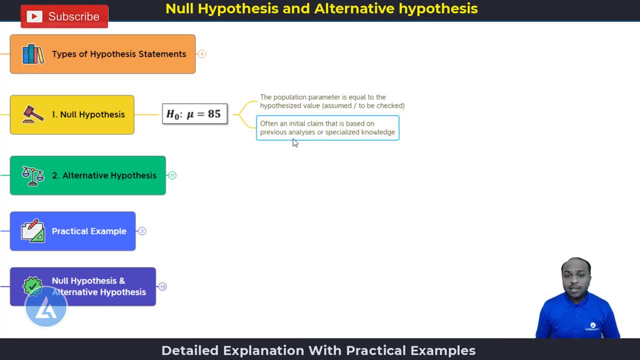 are going to check. This is often an initial claim that is based on the previous analysis or subject matter expert's knowledge. Now let's look at another important statement from this hypothesis testing. This is Alternative Hypothesis. There are three ways to express. 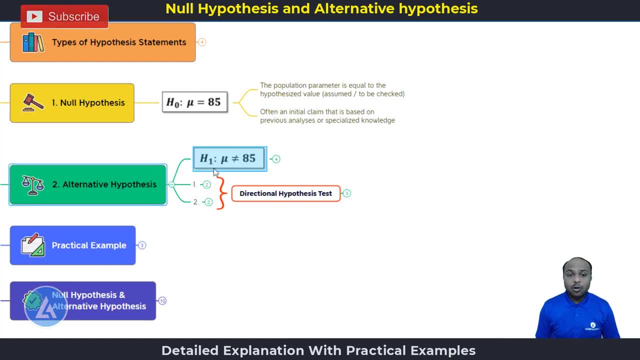 this Alternative Hypothesis. The first one is: H1 colon mu is equal to 85.. The second one is: H1 colon mu is equal to 85.. The third one is H1 colon mu is equal to 85.. The fourth one is: H1 colon mu is not equal to 85.. I will explain this notation in detail. 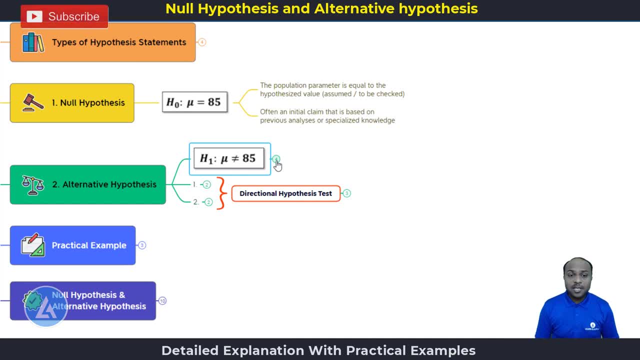 once we go for the example. But just understand, here it is expressed by H1 colon mu is not equal to 85.. The meaning of this notation is: a population parameter is different than the hypothesized value in the null hypothesis. Now this is also called as non-directional. 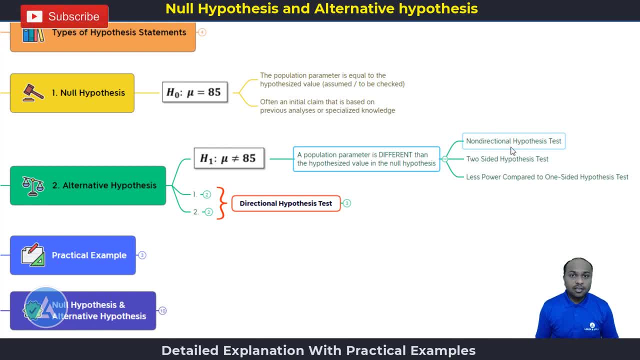 hypothesis test because we are comparing on both sides whether it is less than or greater than. We are just comparing whether it is different than. That's why it is called as non-directional hypothesis test. It is also called as a two-sided hypothesis test. This test is having the less power compared. 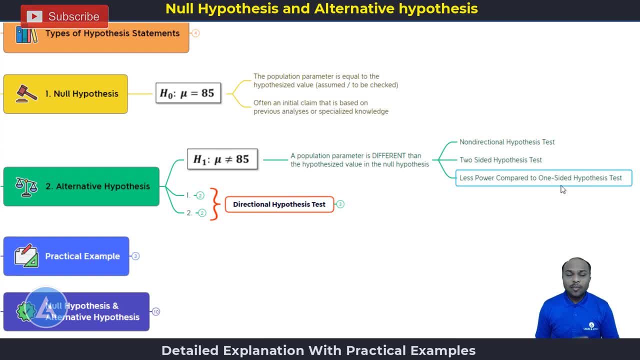 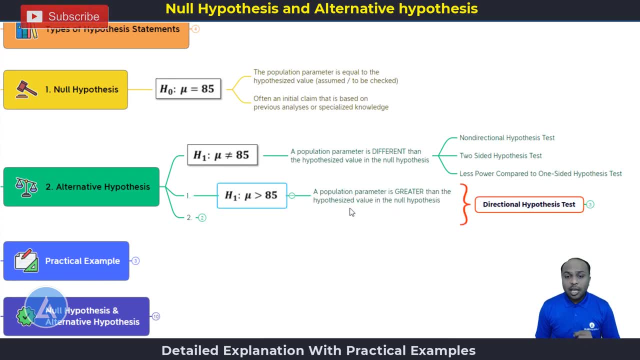 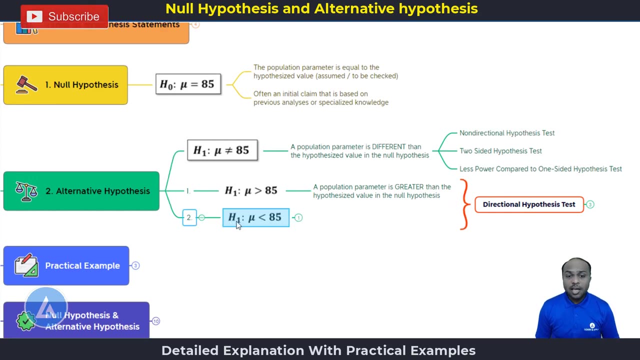 to one-sided hypothesis test. Now let's look at the remaining two statements. H1 colon mu is greater than 85. So this indicates that a population parameter is greater than the hypothesized value in the null hypothesis. And the third statement is: H1 colon mu is: 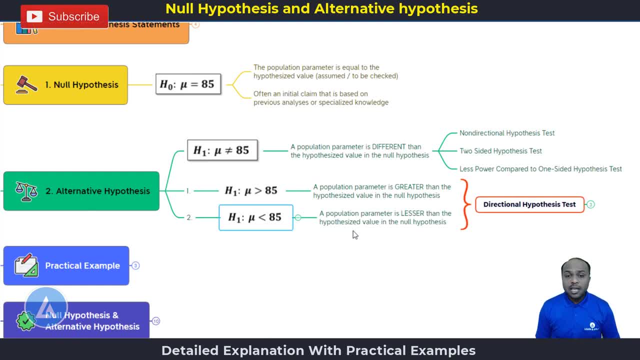 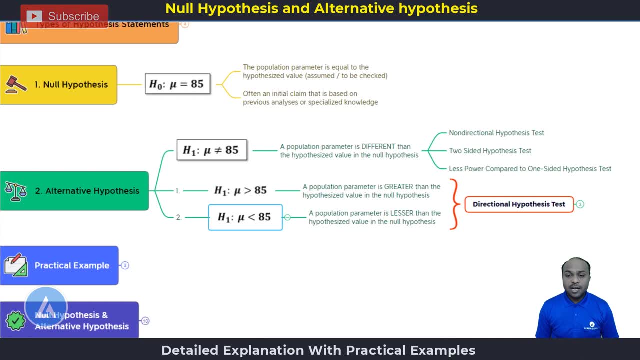 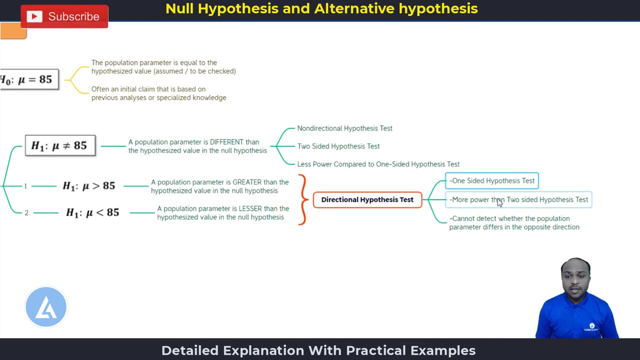 less than 85.. The meaning of this notation is: a population parameter is greater than the hypothesized value in the null hypothesis. Both of these tests are called as a directional hypothesis test. These directional hypothesis tests are also called as one-sided hypothesis test. These are having the more power compared to two-sided hypothesis test, but they cannot. 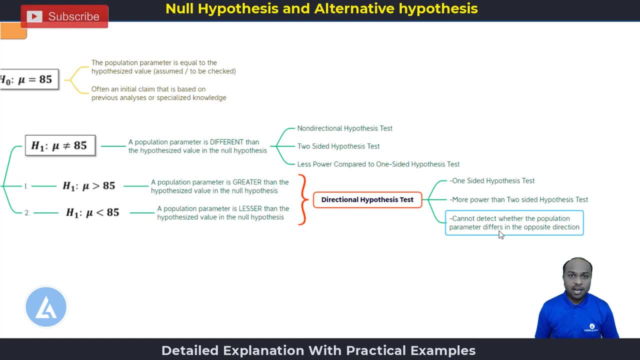 detect whether the population parameter differs in the opposite direction. So, depending on the intent, what we want to check, we need to select any one of these alternative hypothesis. After that, we need to check whether the population parameter is greater than or equal to 85.. 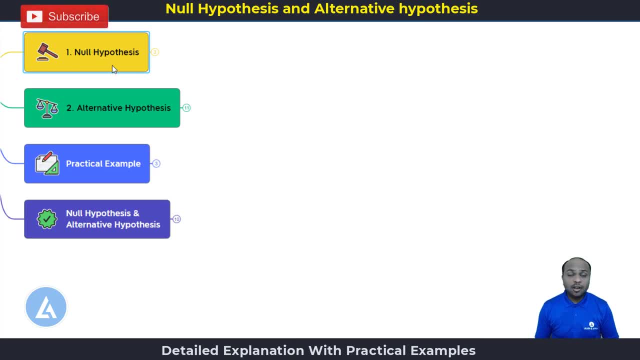 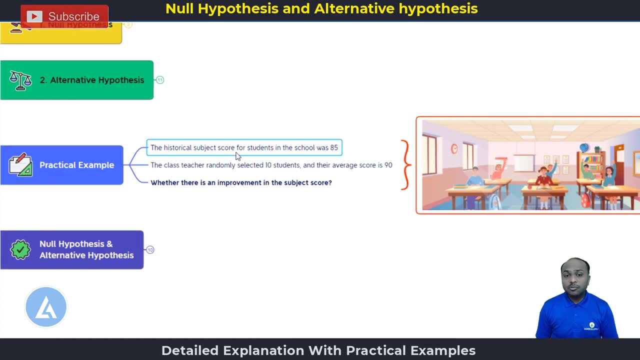 After understanding the theoretical part of this null hypothesis and alternative hypothesis, let's understand them practically. Let's take an example. The historical subject score for the students in the school was 85. But this time the class teacher randomly select the 10 students and take their average. Now, this time the average score is 90. Here. 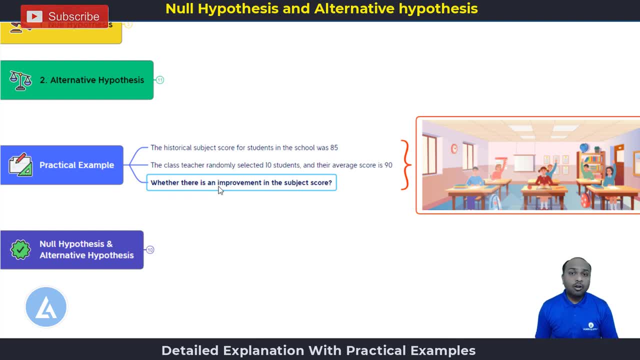 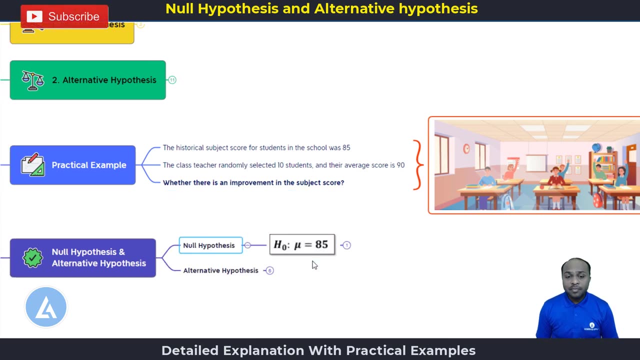 the class teacher wants to check whether there is an improvement in the subject score or not. For that purpose, we are going to use hypothesis testing. Let's understand what is a null hypothesis and alternative hypothesis. in this example, Null hypothesis, as we had seen, it is always in equality and it is indicated by h0 colon. 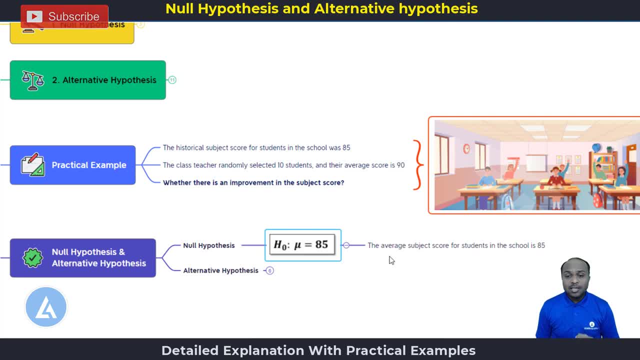 mu is equal to 85.. What is the meaning of this statement? The average subject score for the student in the school is 85. So this is indicating that mean mu is equal to 85.. Now let's talk about the alternative hypothesis. There are three types of alternative hypothesis. 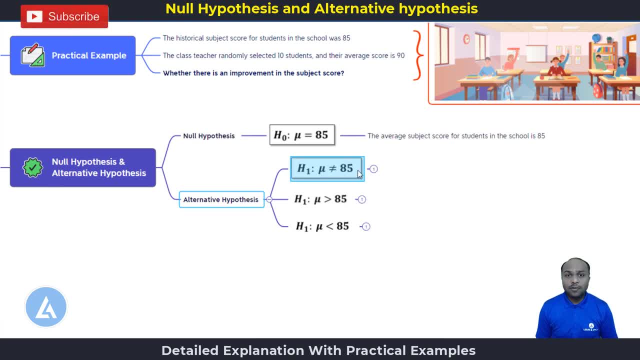 in the school. The first one is: h1 colon mu is not equal to 85. The meaning of this notation is the average subject score for the student in the school is different than 85. Another alternative hypothesis can be: h1 colon mu is greater than 85.. The meaning: